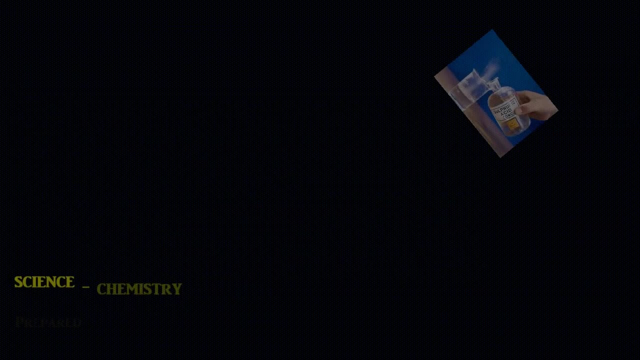 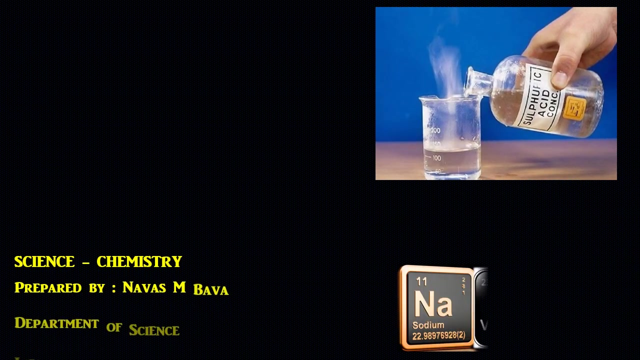 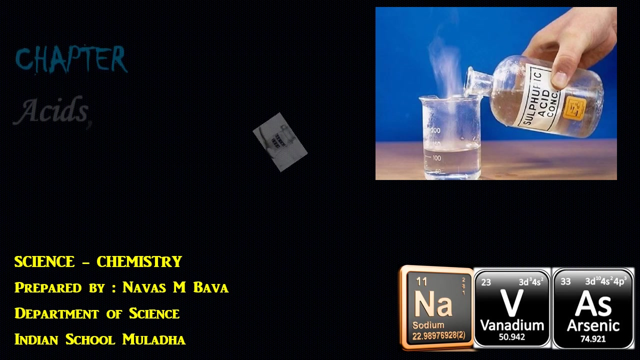 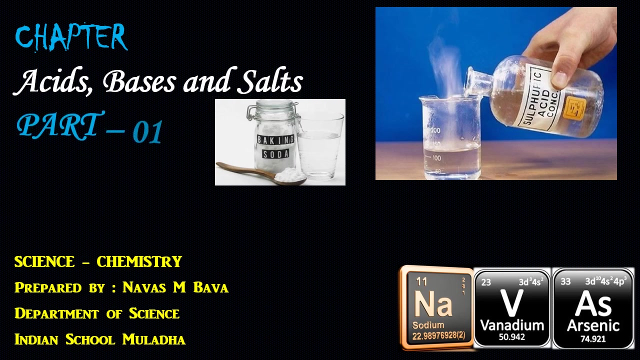 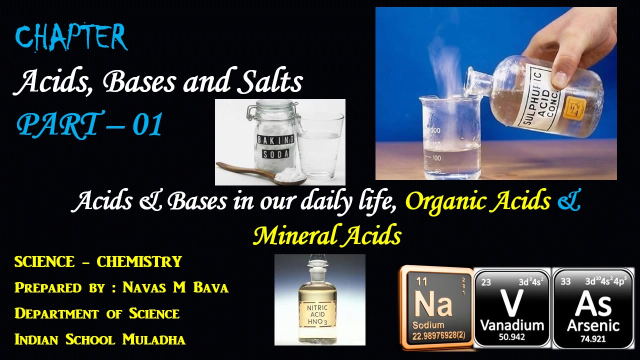 Hello, my dear students. How are you? Hope all are safe and fine at home. This is me, Nawaz M. Bawa. All are welcome to this session. Today, we are going to discuss about new chapter Assets, Bases and Solves. In this presentation, we are going to discuss about assets and bases which we are using in our daily life, especially organic assets and mineral assets. I hope you will enjoy learning with this video. 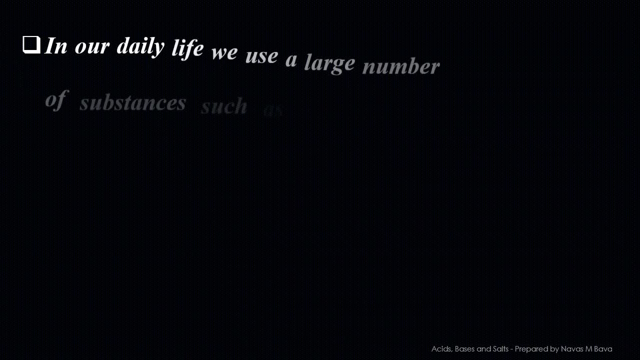 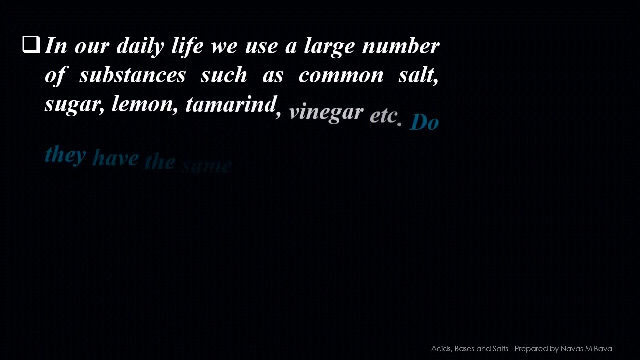 In our daily life, we use a large number of substances such as common salt, sugar, lemon, tamarind. Do they have the same taste? Absolutely no. Different substances are having different 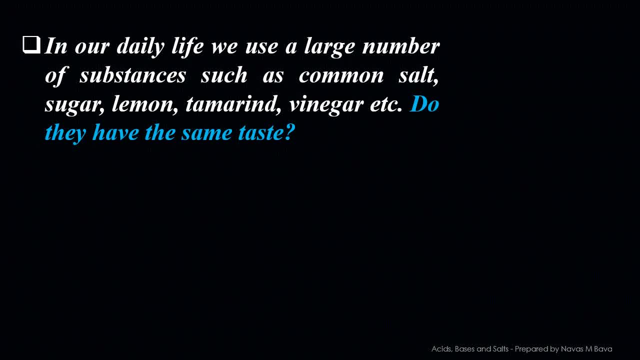 taste. Few examples we can discuss. 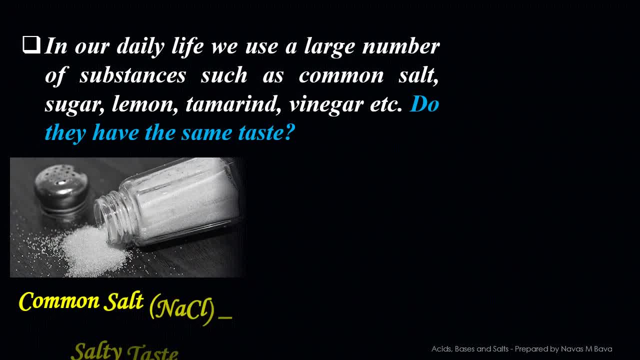 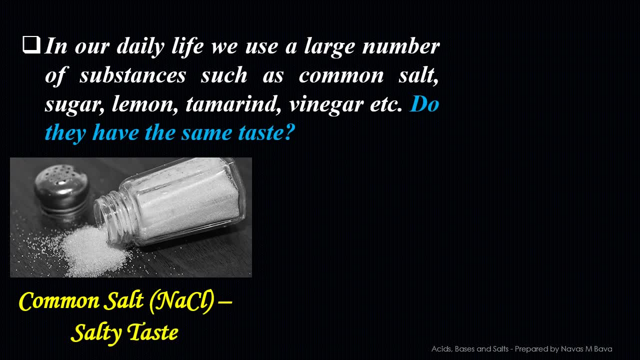 Common salt also called sodium chloride. Chemical formula is NaCl. It is having salty taste. Next one is sugar. Jeannie painting an oil, but I liked this one. 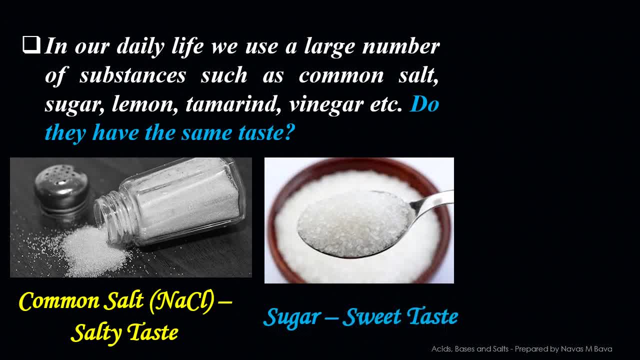 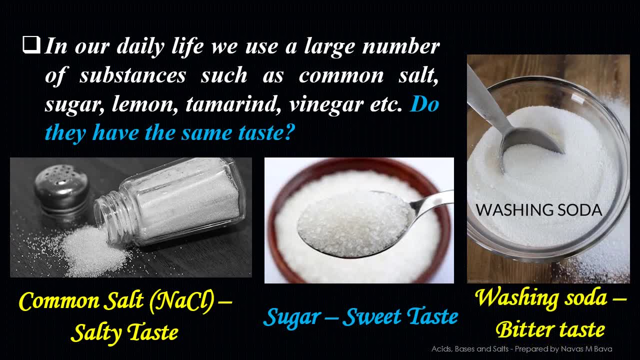 You already know that it has sweet taste. Again another one, we need washing soda. While tasting it, we feel bitter taste. 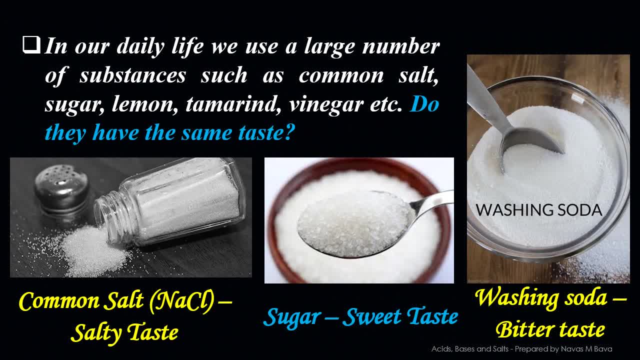 Few more examples we can discuss. Vinegar sour in taste, baking soda bitter taste, or honey in odiggers. We can also add sorghum or sounded, not we. 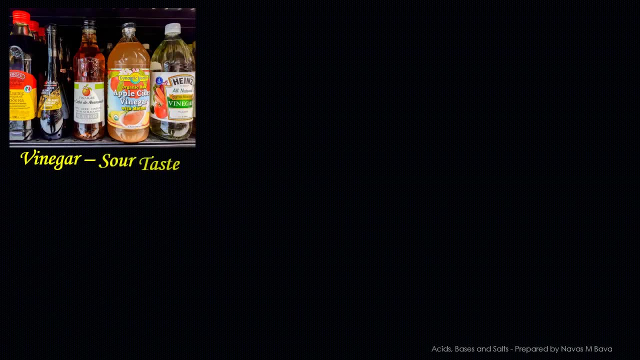 Few more examples we can discuss. Vinegar sour in taste, baking soda bitter in taste, or na financially powdery. You already know that this product has sweet taste. You know this is having a sweet taste. 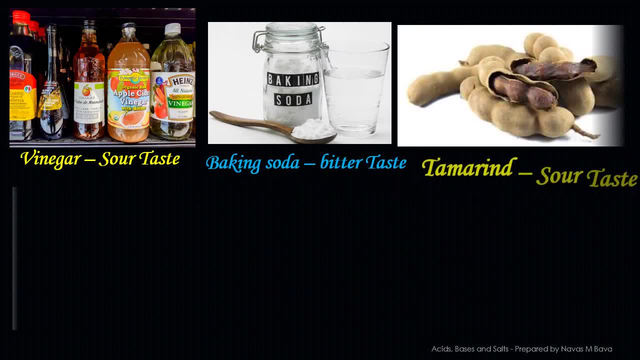 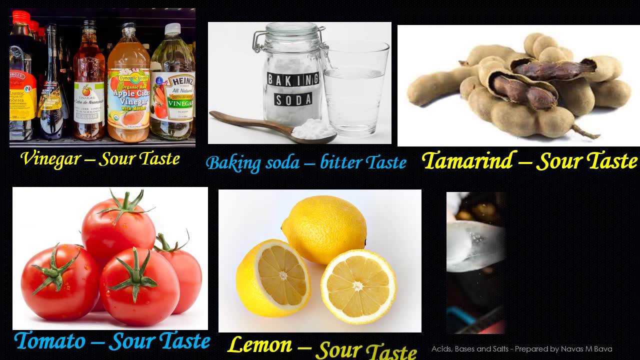 Tamarind So in taste Tomato So in taste Lemon So in taste Soda So in taste 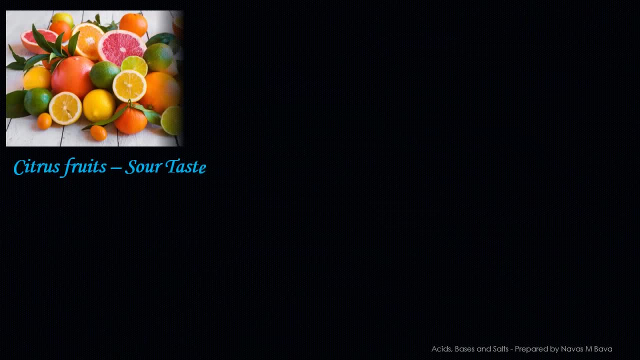 Fruits such as Orange Lemon 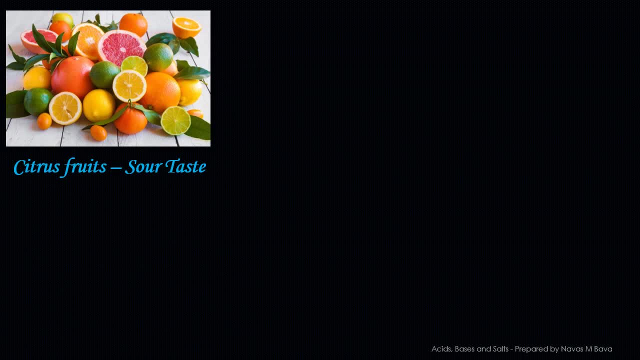 Grapefruit Orange Sweet lemon etc collectively we can call it as citrus fruits 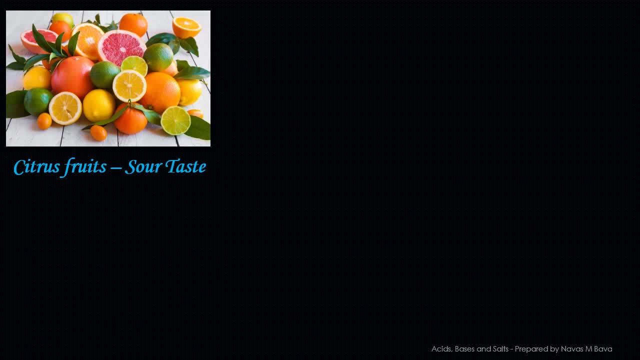 All these citrus fruits are having sour taste in addition with sweet taste Next is apple Apple is in sour taste 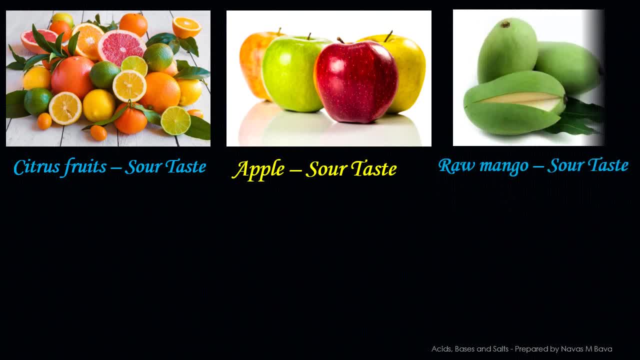 Then Romango It is also having sour taste Next one is amla also known as 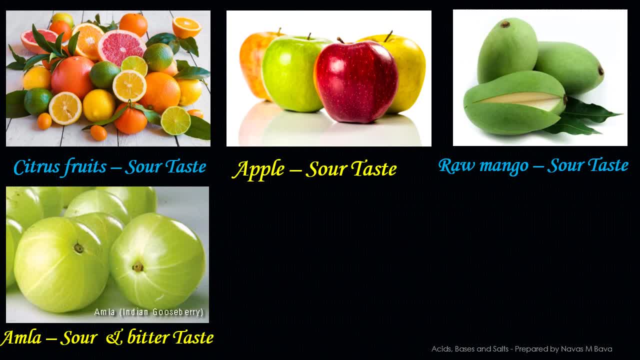 Indian gooseberry It has sour and a little bit of bitter taste 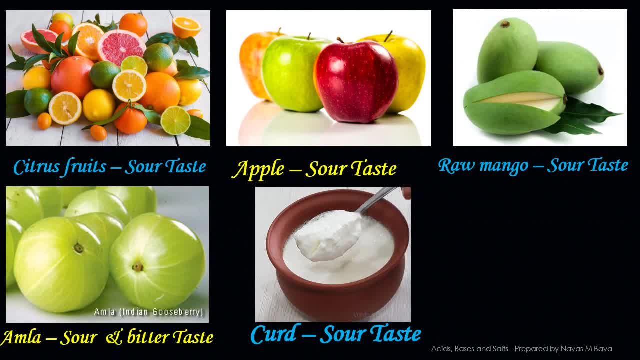 Everyday we are using this curd Curd is having sour taste 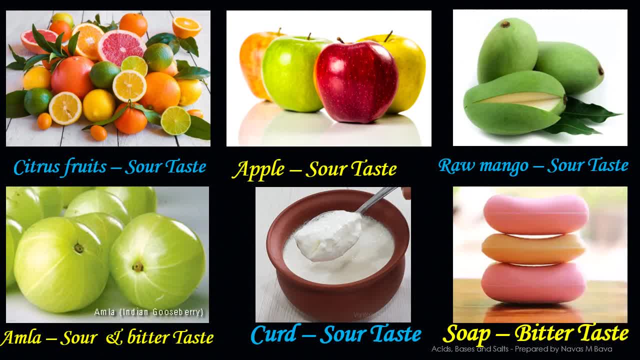 Next is soap Soap is having bitter taste 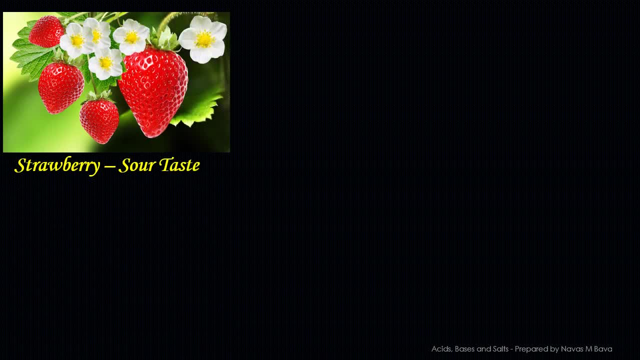 Few more examples Strawberry It has sour taste Then starfruit 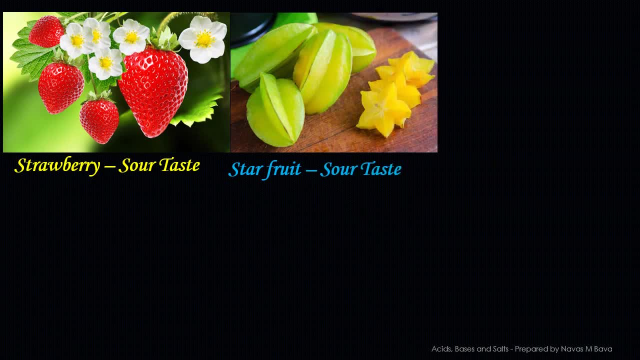 While cutting we will get a star shape It also has Sour taste Next is kiwi It has sour taste 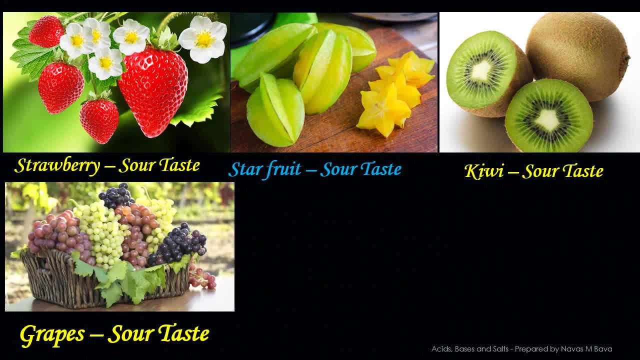 Then different variety of grapes are available It has sour come sweet taste Next is glucose 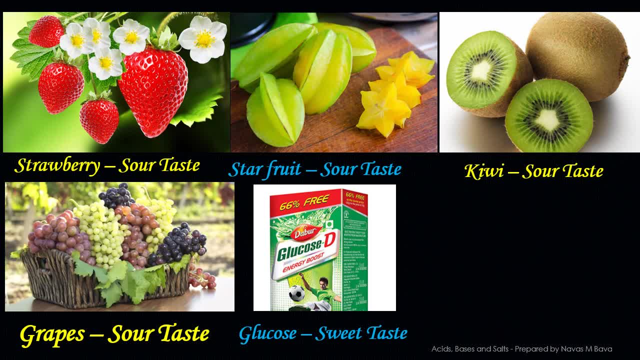 Glucose is having sweet taste 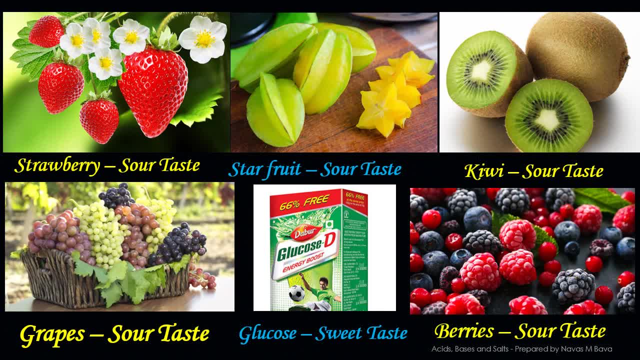 Next different types of berries are available 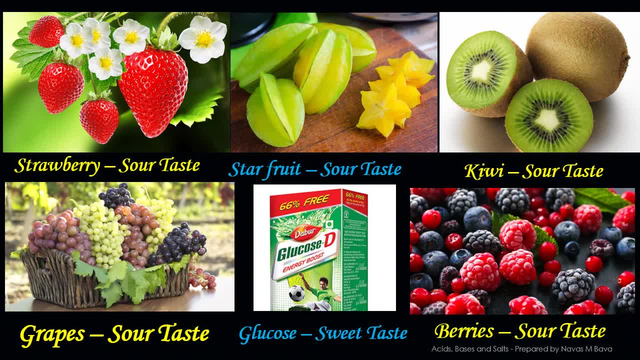 Blueberry, blackberry red berries and all All are having sour taste From these examples 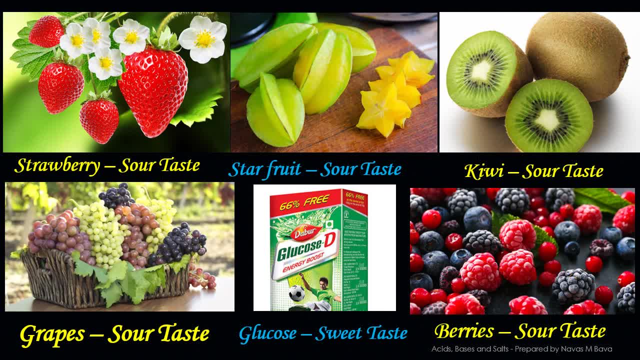 we can understand that different types of fruits vegetables and other substances we are using in our daily life has sour taste and bitter taste and few are having sweet and sour taste 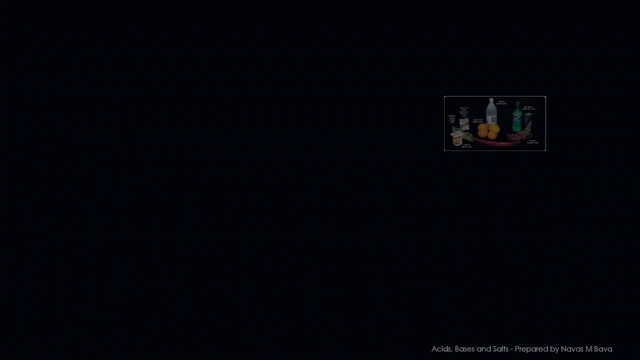 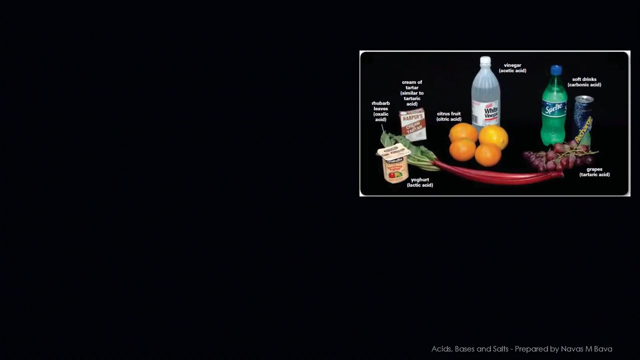 In previous slides we saw examples of different substances with its taste As per taste we can differentiate 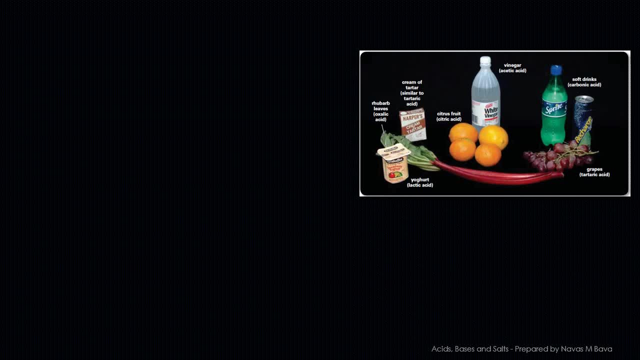 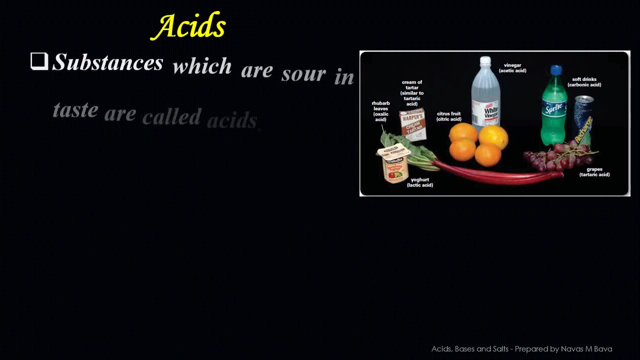 substances into acidic basic or neutral First we can discuss about acids Substances which are sour in taste are called acids 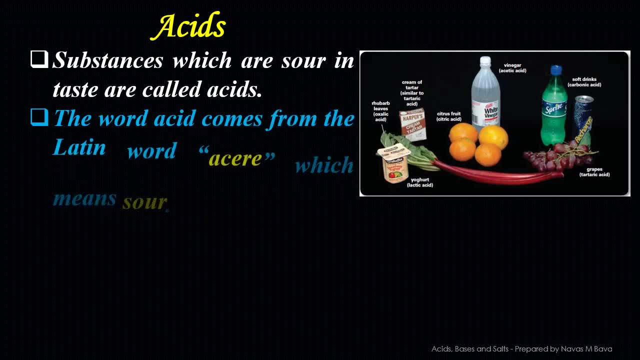 The word acid comes from the Latin word Acere which means Sour 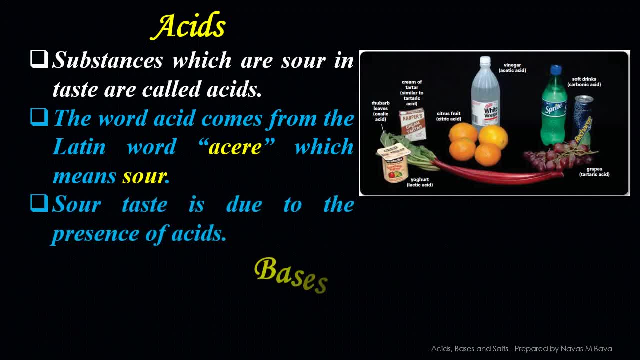 Sour taste is due to the presence of acids 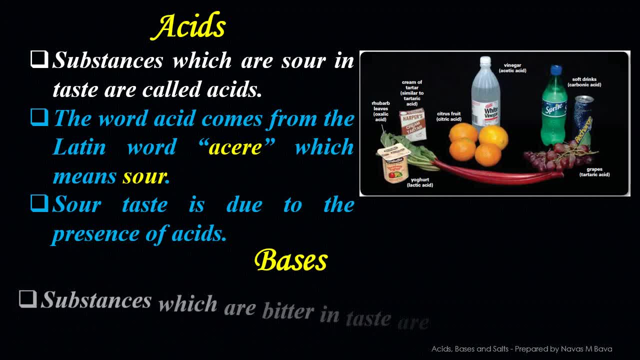 Next we can discuss about bases 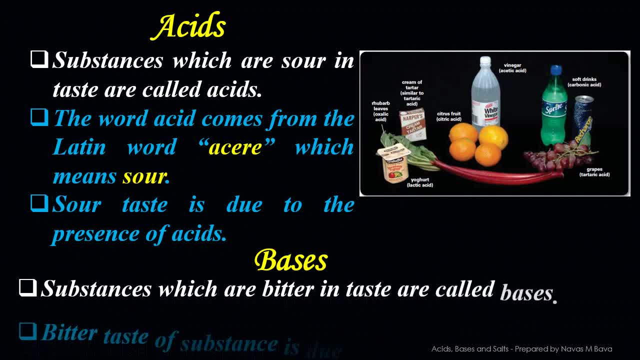 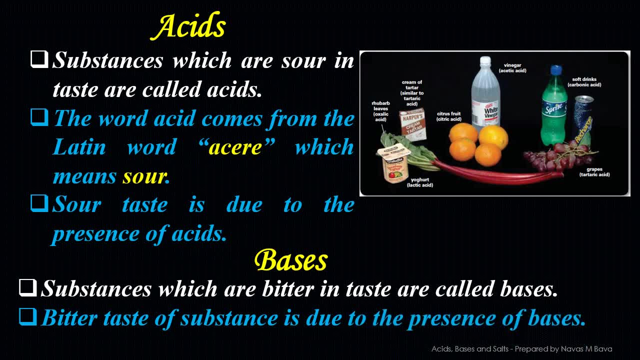 Substances which are bitter in taste are called bases Bitter taste of substance is due to the presence of basic substances 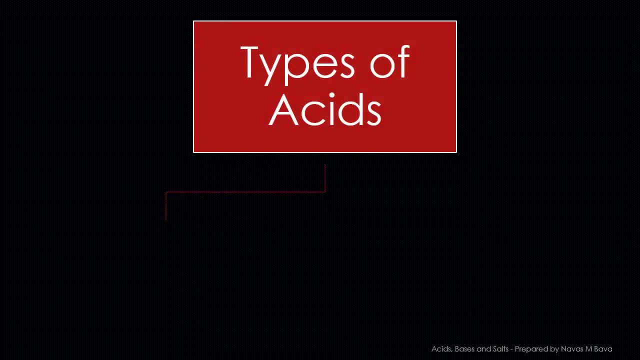 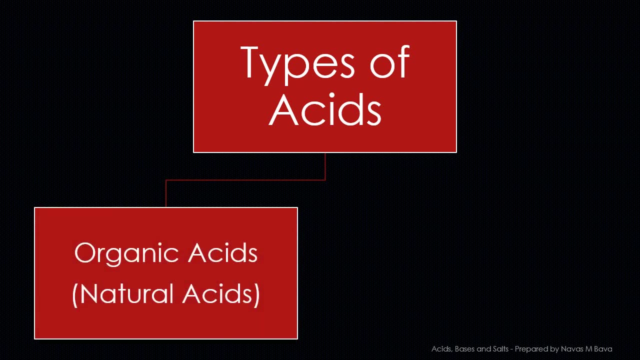 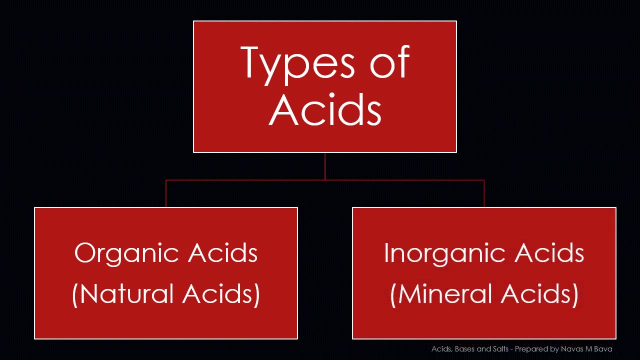 Here we are going to discuss about types of acids Different types of acids are organic acids that means natural acids and the second one is inorganic acids or mineral acids 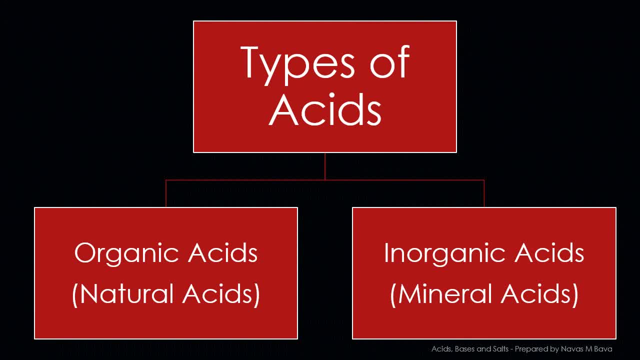 In coming slides we are detailing about these two types of acids 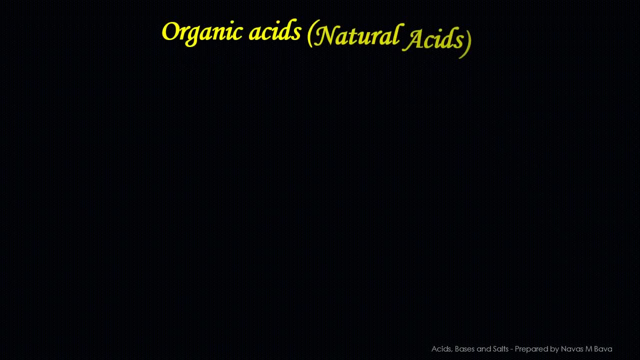 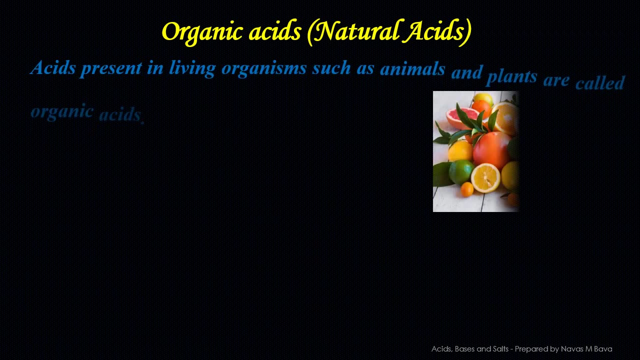 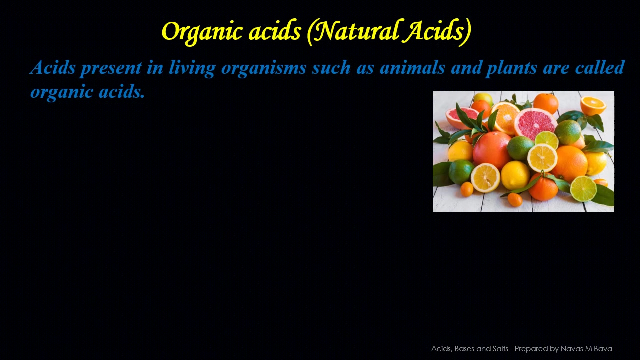 Here we are detailing about organic acids or natural acids Acids present in living organisms such as animals and plants are called organic acids or natural acids Few examples are given below First one is citric acid 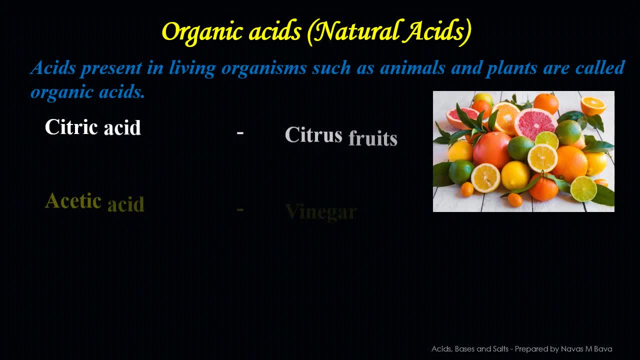 which is present in citrus fruits such as lemon, orange etc Next is 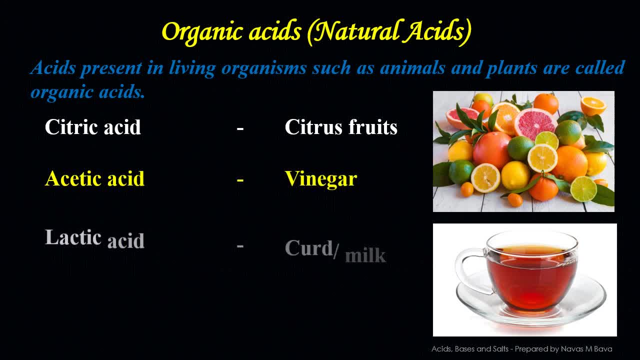 acidic acid which is present in vinegar It is also called ethanoic acid 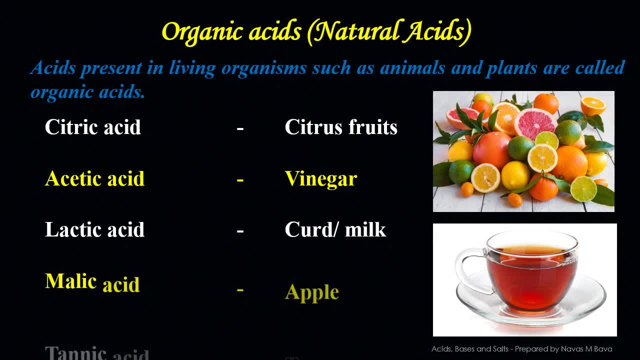 Next one is lactic acid 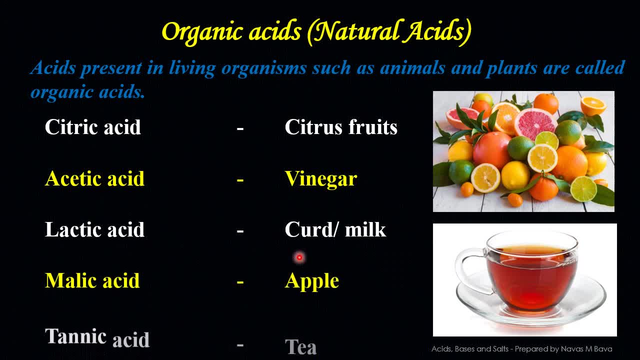 which is present in curd or milk Next is 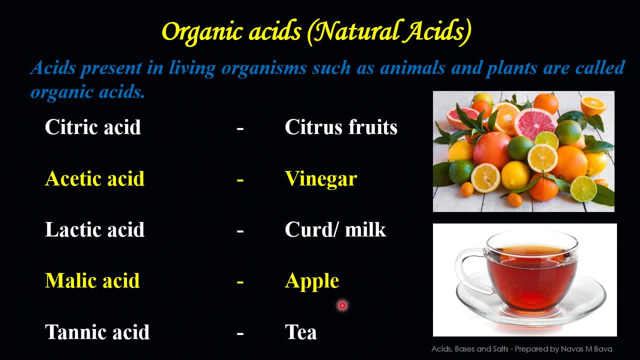 malic acid which is present in 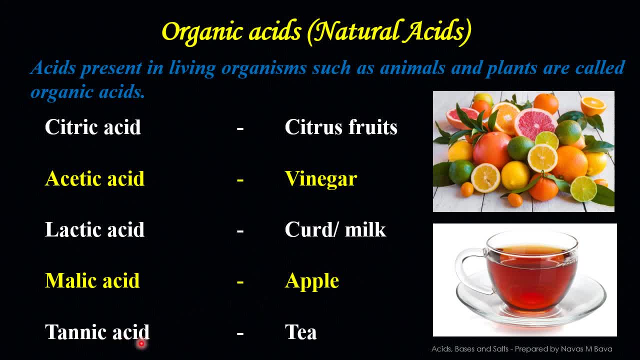 apple Next is tannic acid present in tea and also coffee 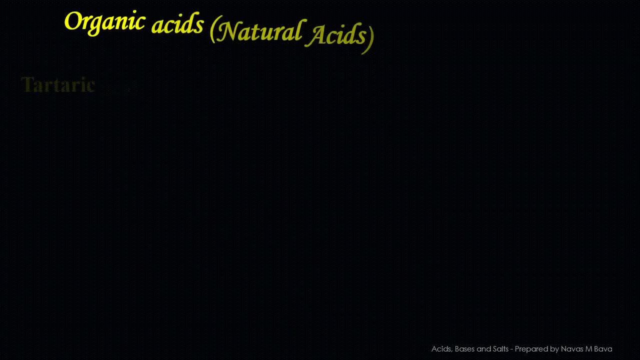 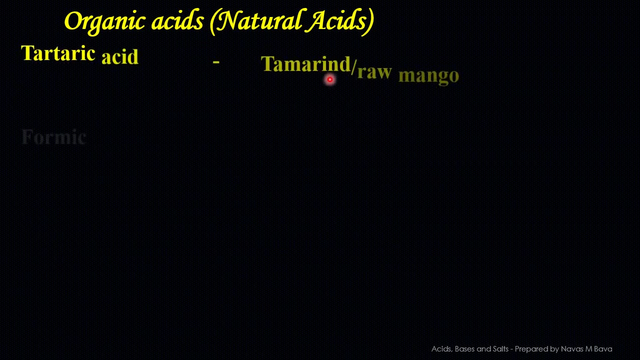 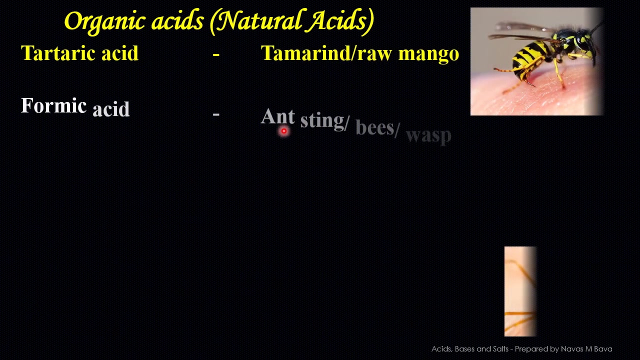 Few more examples of organic acids or natural acids are tartaric acid which is present in tamarind and also raw mango Next one is formic acid which is present in ant sting or bees or wasp 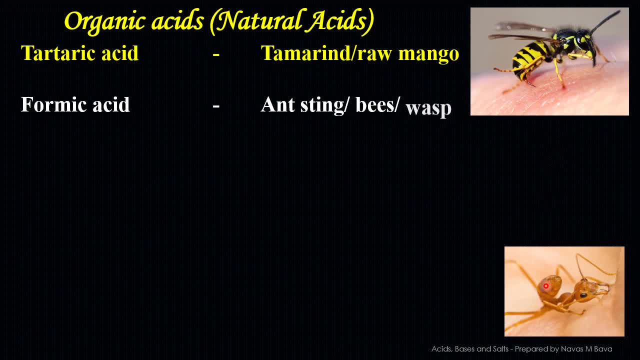 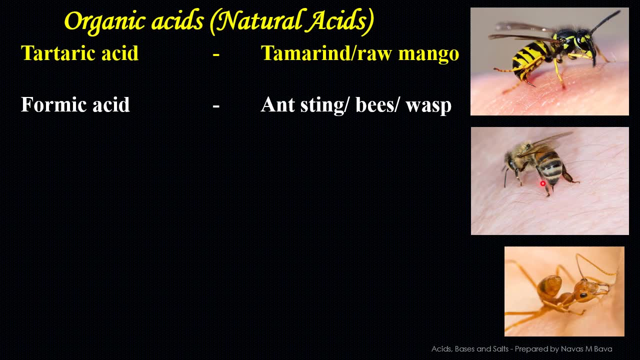 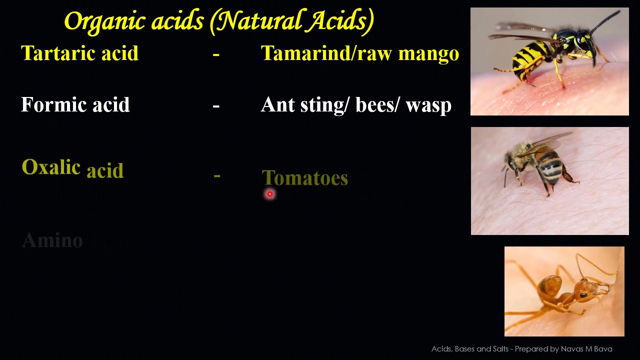 Then ant stings or bees or wasp stings it injects formic acid another name is methanoic acid Next one is oxalic acid which is present in tomatoes Next one is amino acid that is present in proteins Next one is 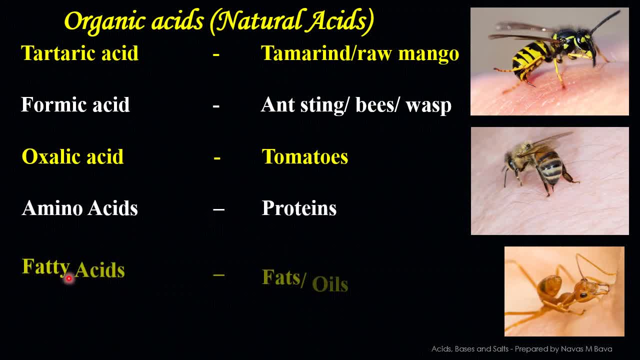 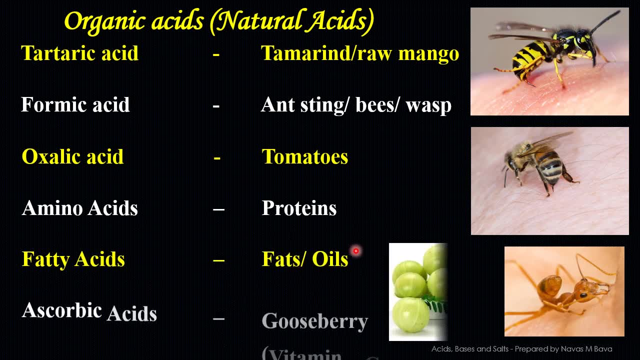 fatty acids which is present in fats and oils like as our sunflower oil coconut oil mustard oil etc